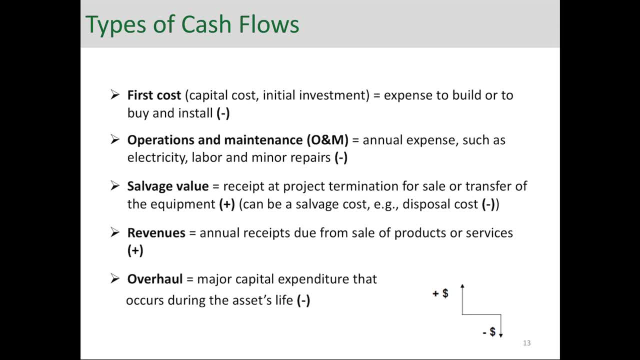 that you pay to buy an asset or any kind of machine, Any costs and that's a negative cash flow. Operations and maintenance costs: Those are overtime and regular expenses to maintain an investment and typically you know electricity labor or any minor repairs that you pay for them regularly. Those are also costs. 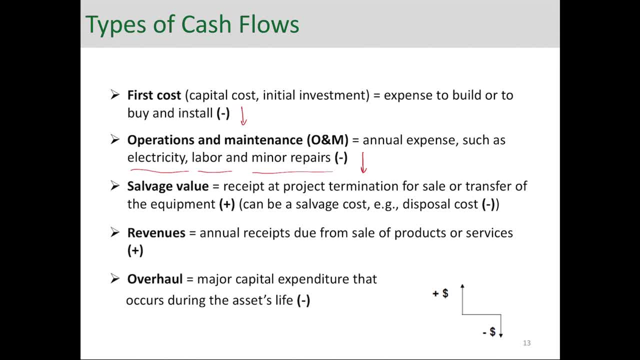 So negative cash flows. Salvage value: That's the value of an asset at the end of its life. It's typically positive because you can sell that asset for some money and that's a salvage value. But it can be also negative if that asset needs a disposal cost. 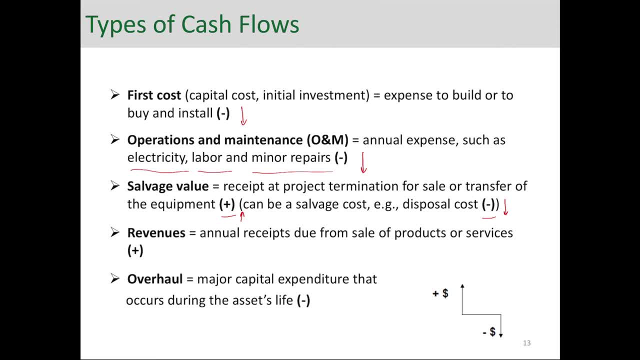 Basically, you need to pay in order to get rid of it. We also have revenues. Those are positive cash flows due to, you know, sales or anything positive cash flow that your business generates. So those are positive cash flows. You also have typically overhaul costs. sometimes Those are major expenses due to 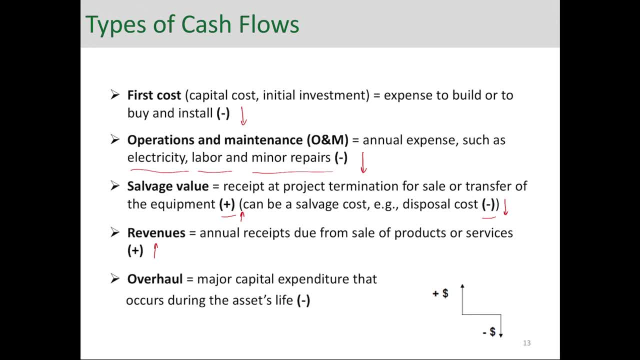 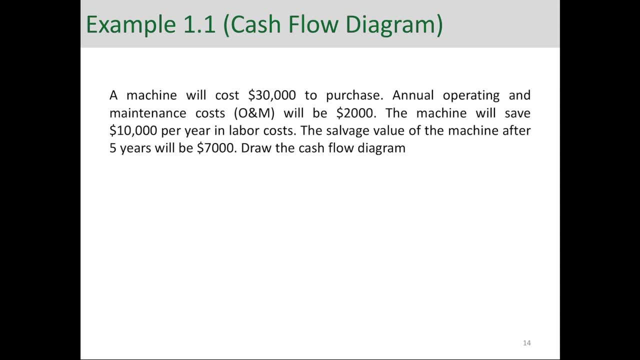 a sudden repair or something. Let's look at this simple example and draw a cash flow diagram for it. A machine will cost thirty thousand dollars to purchase. Operating and maintenance costs will be two thousand. The machine will save ten thousand per year in labor costs. 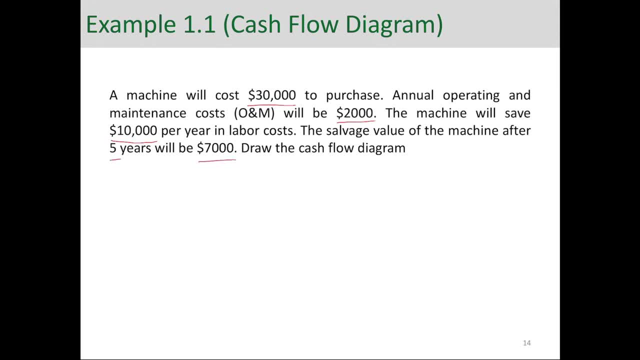 The salvage value of the machine after five years will be seven thousand. Draw the cash flow diagram. So let's start with the time horizon here And as you can see, it's over five years. So year one, two, three, four and five. 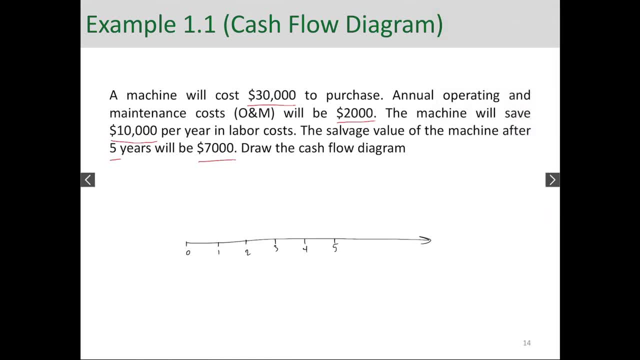 The initial investment is thirty thousand dollars, So that's a negative thirty k. Then annual operating and maintenance costs will be two thousand dollars each year, So some two thousand dollars cash flows over five years. The machine will save ten thousand dollars per year, So that's a 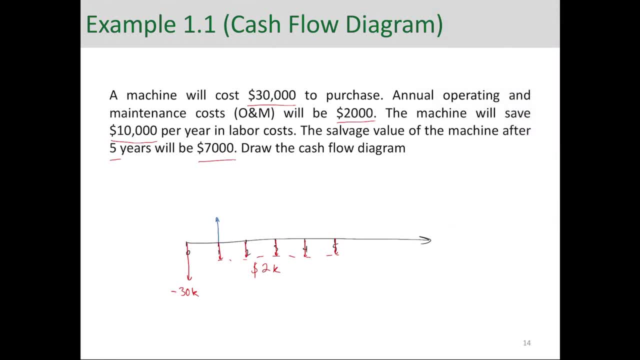 savings. So that's a positive cash flow. So we have some ten thousand dollars here Again over ten years, So ten k, And then there is a salvage value at the end of year five for seven thousand dollars. So at the end of year five we have additional.